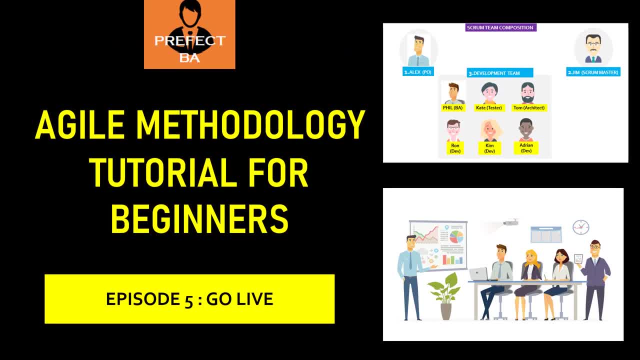 Welcome to Episode 5 of the Agile Methodology Tutorial for Beginner Series. If you have not checked out the earlier episodes yet, please use the links in the description box to check it out before you watch this episode Story. so far, Jane wanted a home delivery mobile app for her restaurant Wagon Gardens. 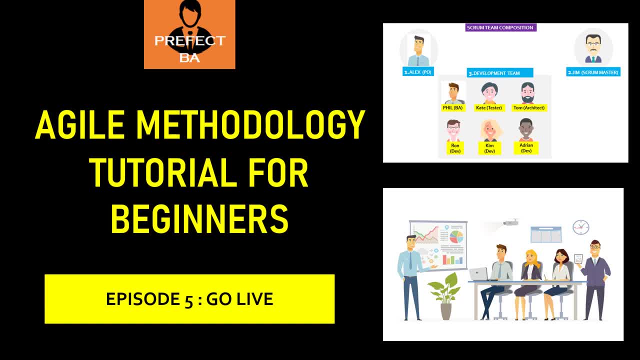 Jane works with WebWeave, an app development company, to get this app developed using Agile methodology. High level requirements were gathered, requirements were prioritized for MVP- ie Minimum Viable Product- and the Scrum team was onboarded and all the required tech tools and environment setups were done as part of Sprint 0. 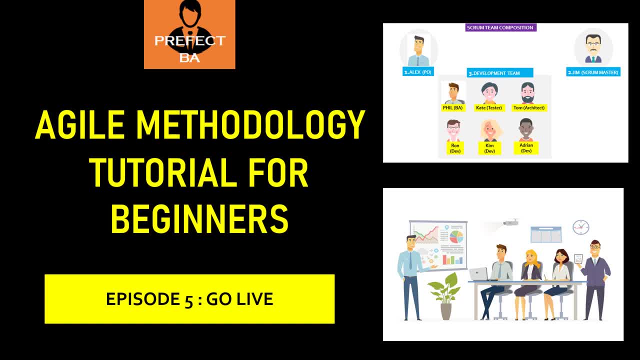 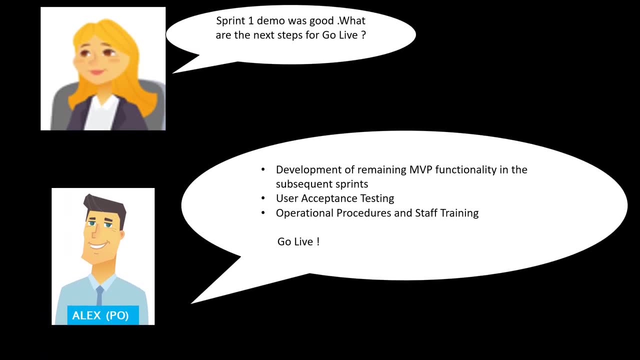 and we looked at different events or ceremonies which were part of a Sprint and product increment was showcased In this episode. we will conclude the story with the Go Live of the mobile app. Jane was very happy with what she saw as part of Sprint 1 demo. 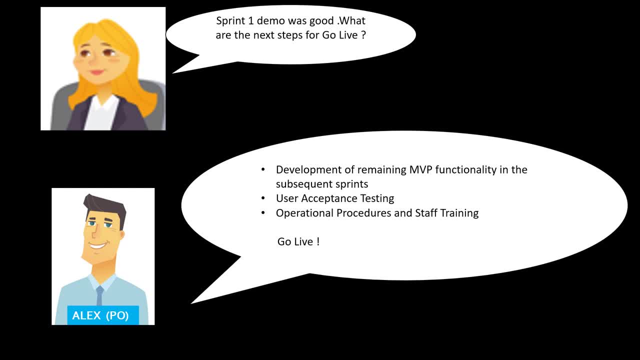 She asked Alex: Sprint 1 demo was good. what are the next steps for Go Live? Alex was happy to hear Jane's feedback and then he mentioned that there were three key activities before Go Live: 1. Development of remaining MVP functionality. 2. Development of remaining MVP functionality. 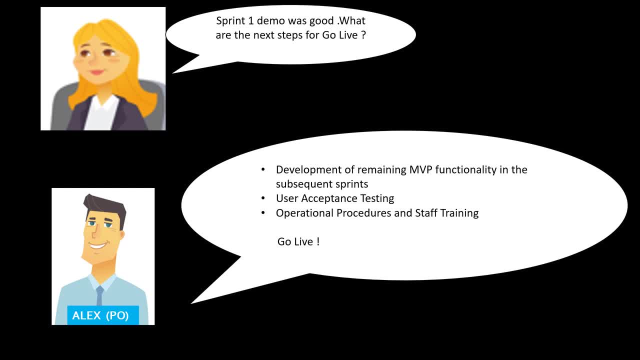 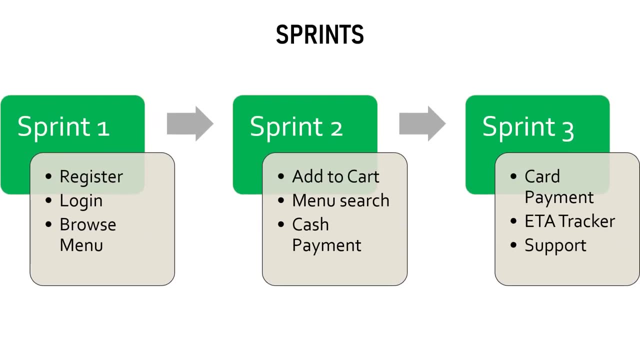 in the subsequent Sprints: 2. User acceptance testing, 3. Operational procedures, creation and staff training, and then Go Live. We will cover each of these activities in the subsequent slides. As we saw in the previous episode, Sprint 1 delivered the three functionalities. 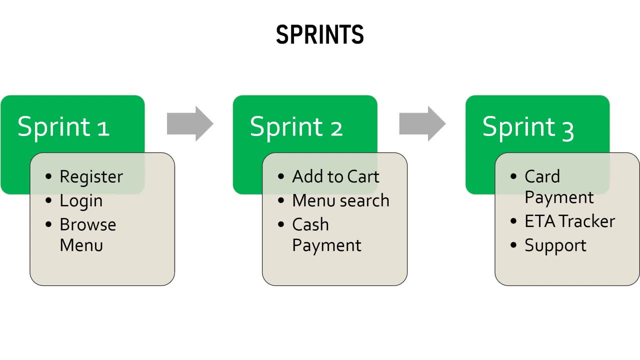 Register, Login and Browse feature for food items in the menu. The team continued the same process involving the five Sprint ceremonies for each of the subsequent Sprints. Sprint 2: delivered. add and remove to the cart functionalities. menu search for customers. to search for food items. 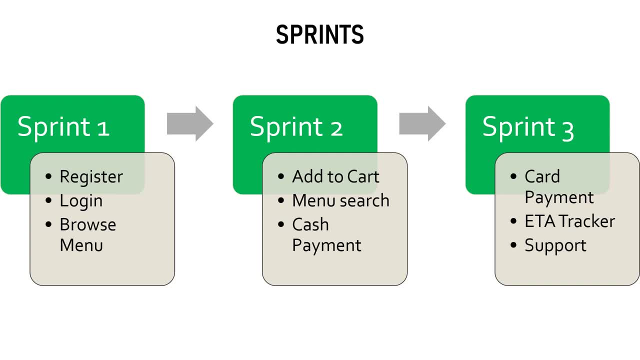 and also feature of accepting cash on delivery from the customer. Sprint 3 delivered, customer's ability to pay using debit or credit card, expected time tracker for the food to be delivered and the customer support feature for any issues faced by the customers. These functionalities were showcased as part of the Sprint demos to Jane and her team. 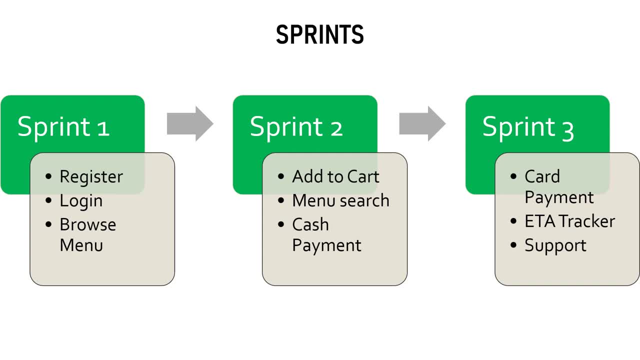 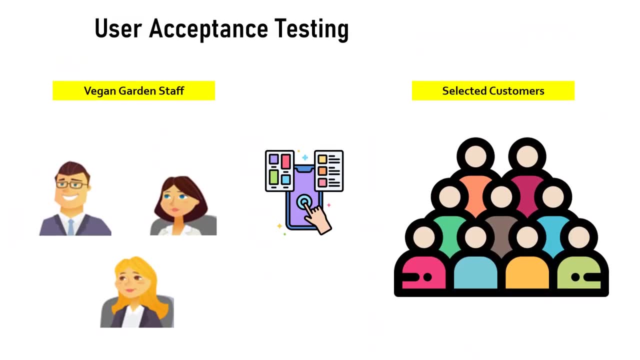 They were very happy with the functionalities showcased and the minimum viable product features had been developed and was ready As all the features decided for MVP had been developed. the next step towards Go Live was User Acceptance Testing, or UAT. Alex's team made the application available for UAT. 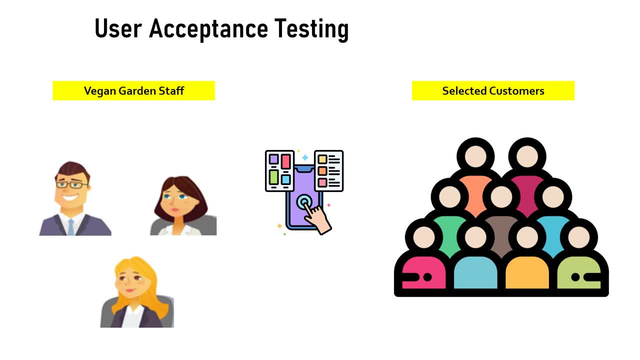 There were two sets of people who were performing the test. First one Wagon Garden staff. They checked the developed functionalities and ensured that the app was customer friendly. They also focused keenly on the staff side of the application, That is, whether they were receiving the orders properly. 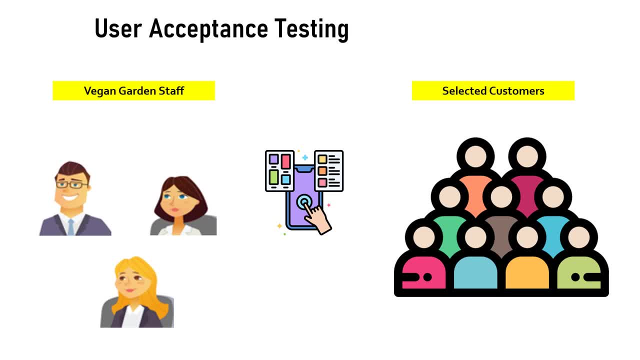 online payment was showing up in their business' current account and whether they were able to receive and respond back to the customer. The second set of audience for testing were the selected customers who visited the restaurant regularly. Jane requested for their help on reviewing the application and requested feedback. 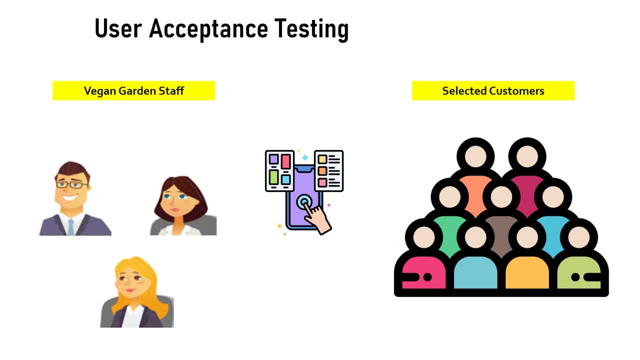 These customers checked whether the app was easy for navigation and ordering and if there were any issues during the booking process. The defects identified during the testing process were fixed by the Scrum team. New features and feedbacks were added to product backlog as a user story. 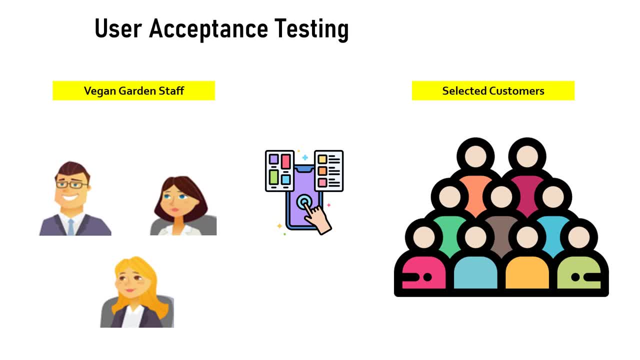 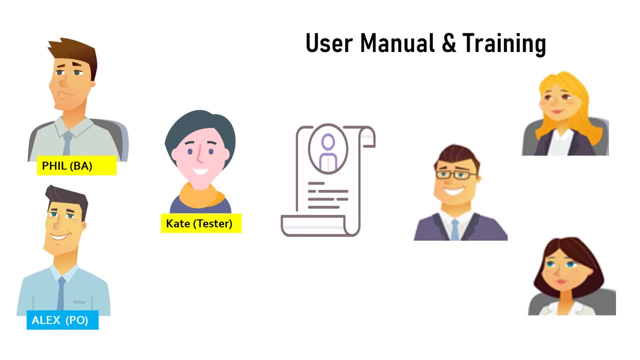 by Alex and Phil for prioritization later on. While the UAT is going on, another activity which is done in parallel is drafting of user manual and staff training. Phil and Alex worked on creating a user manual with details of the developed functionalities and step-by-step instructions for usage of the app. 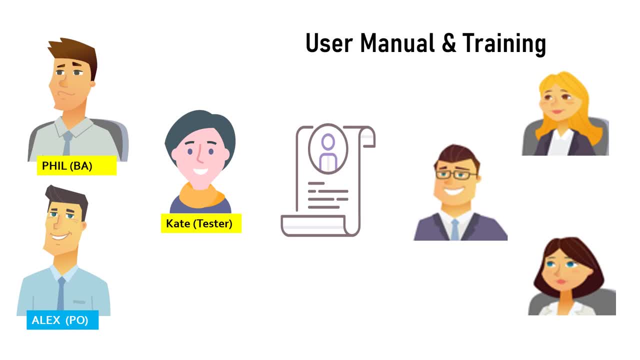 This would be the go-to guide for the staff to start using the application and also to refer for any issues in the future. Also, Kate and Phil provided live training sessions to make them familiar with the user interfaces and functionalities. MVP functionalities were developed.